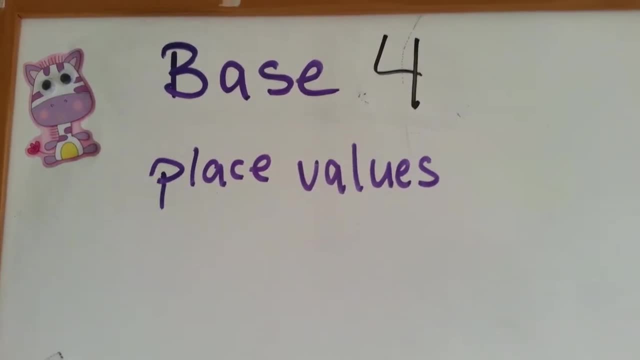 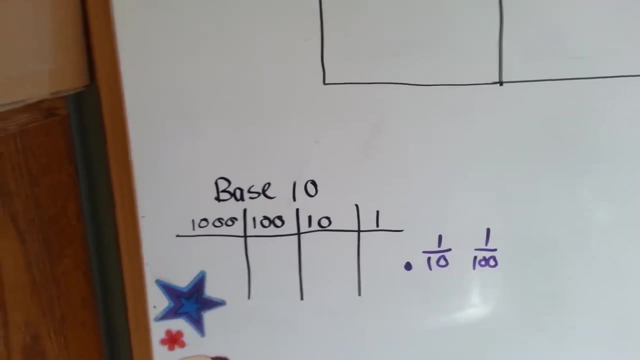 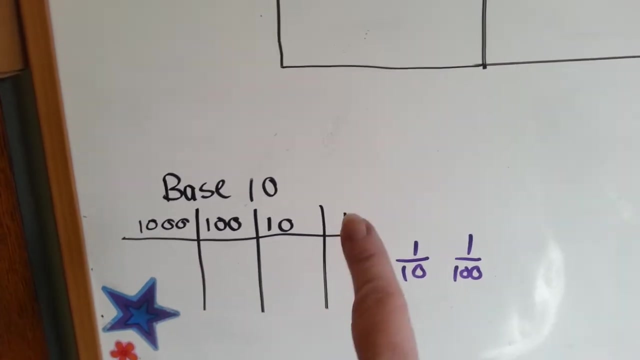 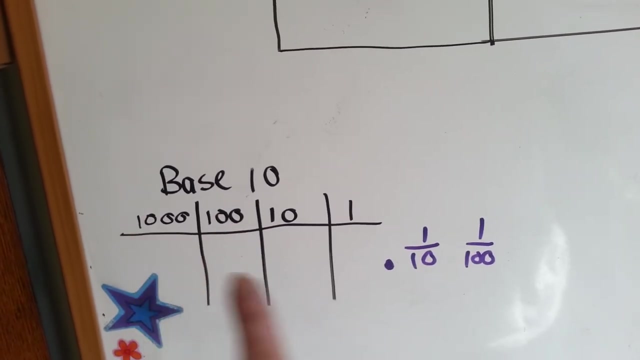 Base 4, place values. We're doing base tables Now. in our normal everyday world we work off of base 10.. Base 10 is: every time you go to a place value to the left, you multiply it by 10.. 1 times 10 is 10.. 10 times 10 is 100.. 100 times 10 is 1,000.. And we keep going that way, multiplying by 10, to get to our next column. 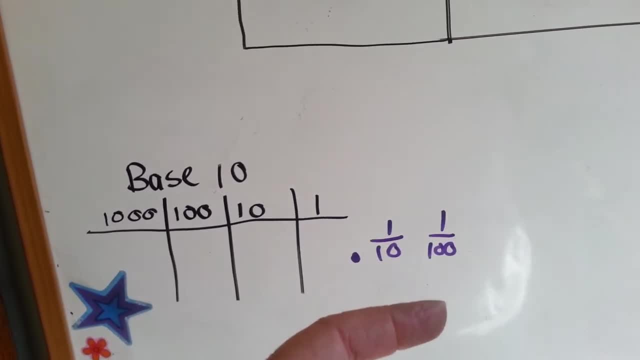 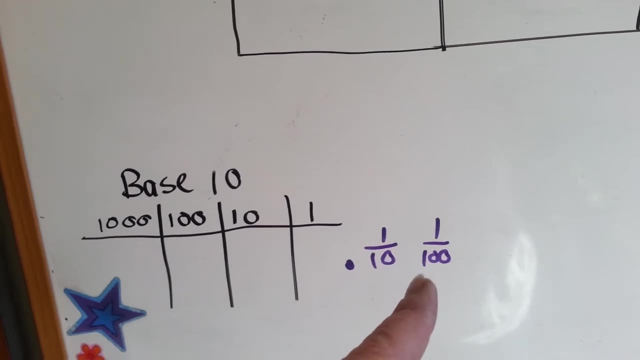 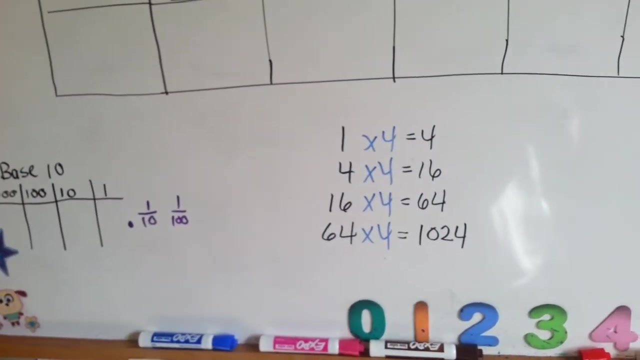 And then on this side, to the right of the decimal point, we divide by 10.. So the first place value here would be 1 tenth, And then the next one here would be 1 one hundredth. Well, in base 4, we're multiplying, except not by 10,, like the base 10 does. we're multiplying by 4. And that tells us right here what our columns are going to be. 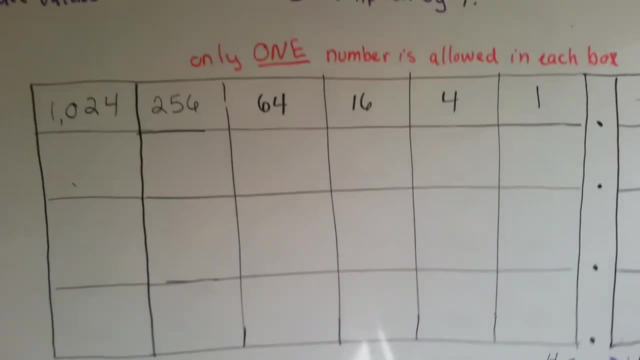 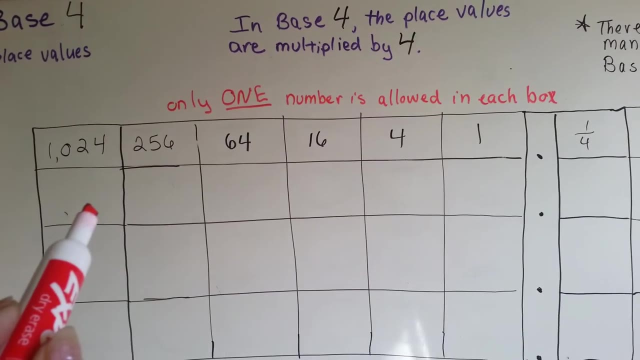 This is what our place value columns are going to be. So let's take a look. So each place value is multiplied by 4.. So each place value is multiplied by 4.. We're only allowed to put one number into each box. 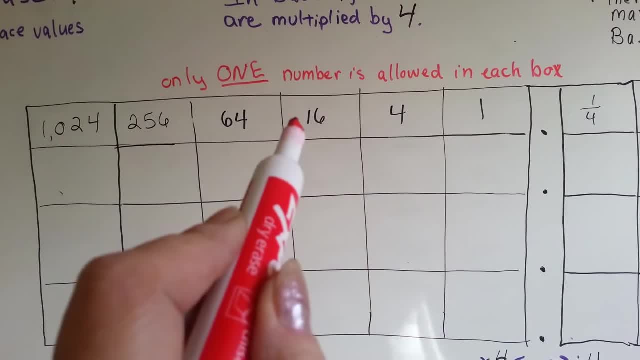 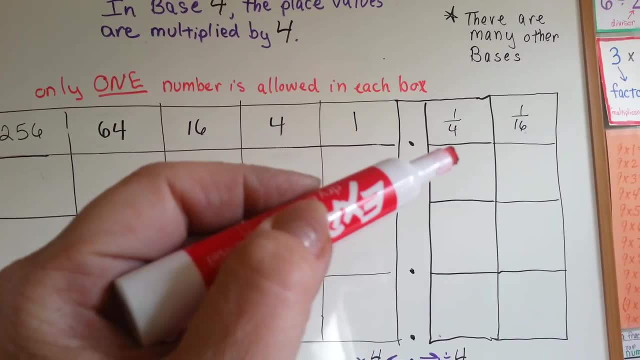 So we go from 1's to 4's, to 16's, to 64's, to 256's, to 1024's, And then to the right of the decimal place, we have 1 fourth's and 1 sixteenth's. 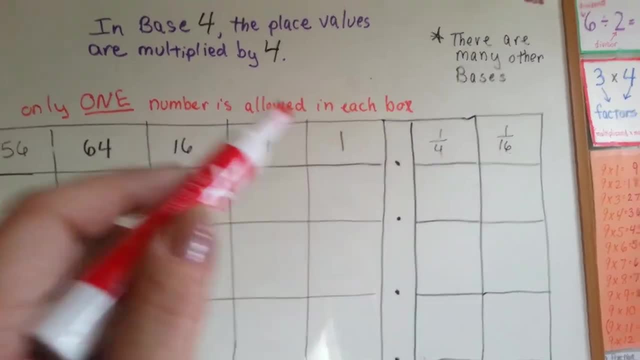 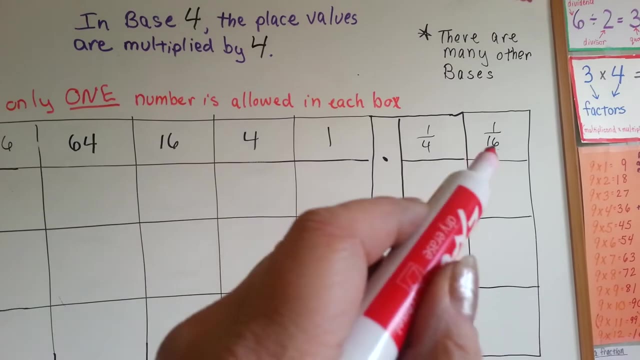 Now, normally that would be the 10th's place, wouldn't it? And that would be the 100th's place, But because we're in base 4, it can't be bigger than 4.. Okay, And 4 times 4 is 16.. 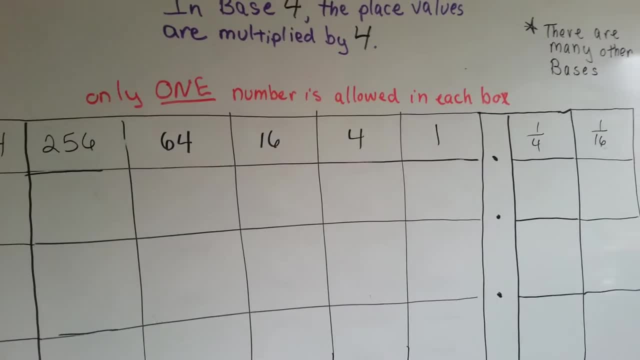 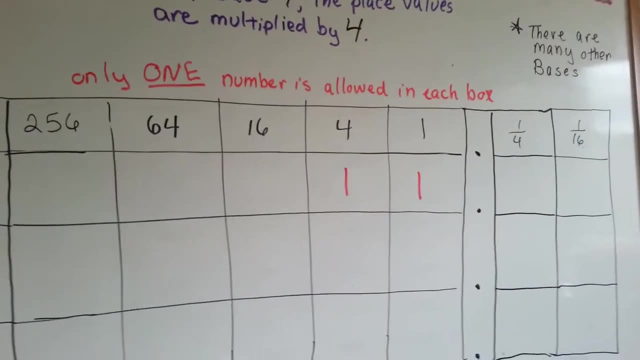 So that's 1.. So if I wanted to write the number 5, I would have to put 1- 4 and 1- 1. And that would make 5.. So in base 4, an 11 would really be 5.. 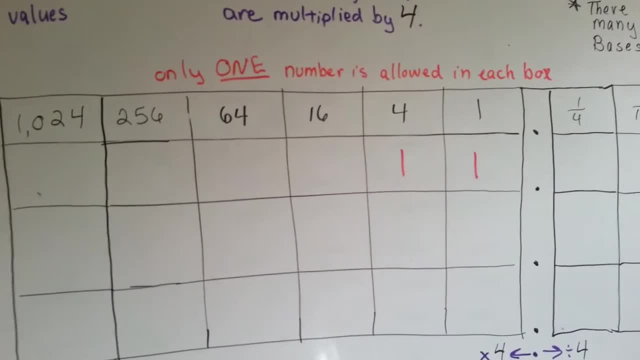 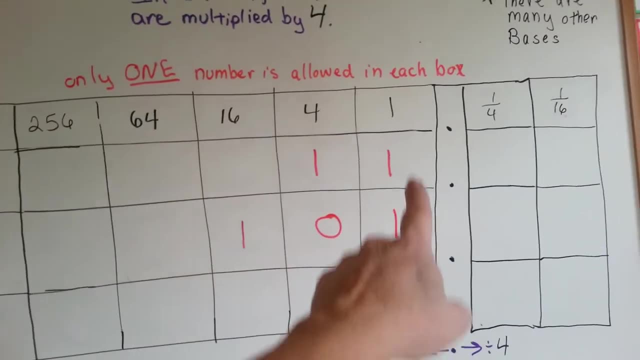 Is that confusing? Check this out. How would you write 17?? You'd have 1, 16, no 4's and a 1. That's how you would write the number 17.. See How would you write the number 66?.